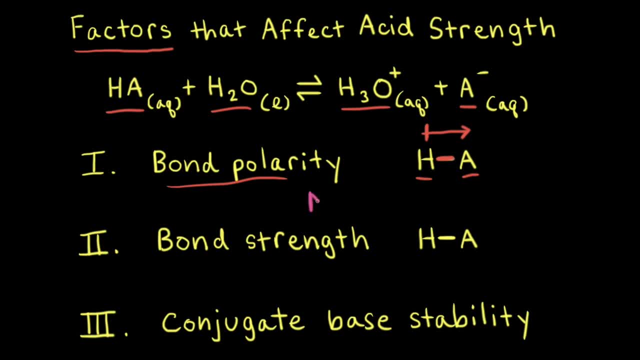 are pulled closer to the A. As the electronegativity of A increases, there's an increase in the polarity of the bond. As the bond polarity increases, more electron density is drawn away from the H, which makes it easier for HA to donate a proton. 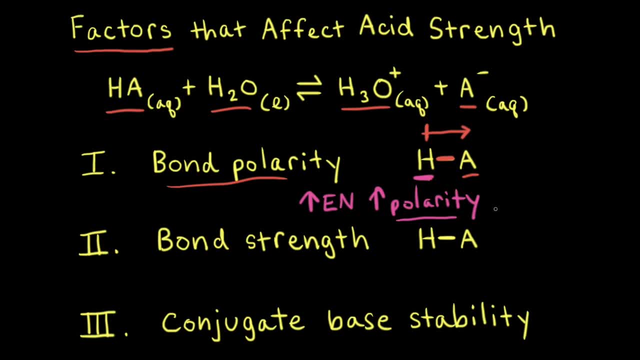 Therefore, in general, an increase in the polarity of the HA bond means an increase in the strength of the acid. Next, let's think about the factor of bond strength and let's consider the strength of the bond between H and A. The weaker the bond. 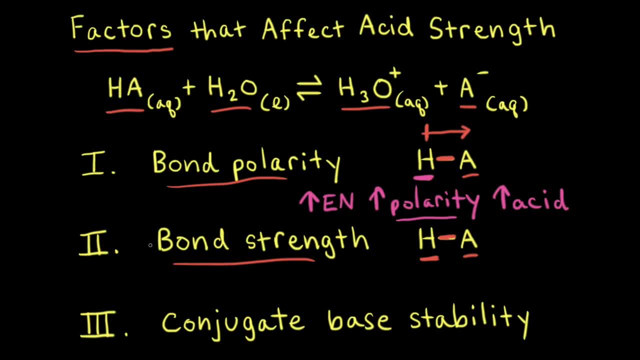 the more easily the proton is donated. Therefore, in general, a decrease in the bond strength means an increase in the strength of the acid. The stability of the conjugate base can also affect the strength of the acid. The more stable conjugate base, the more likely the acid is. 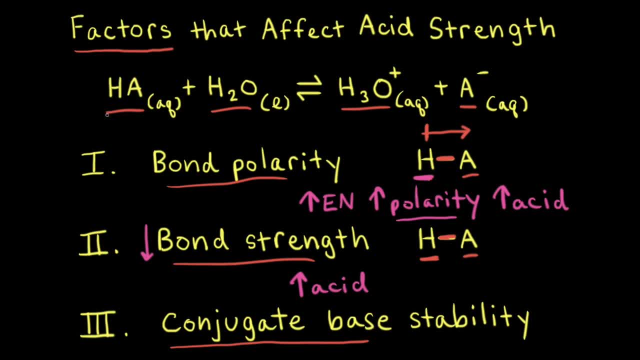 to donate a proton. So if you think about that, for HA the conjugate base is A minus And the more stable A minus is, the more likely HA will donate a proton in solution. Therefore, in general, the more stable the conjugate base. 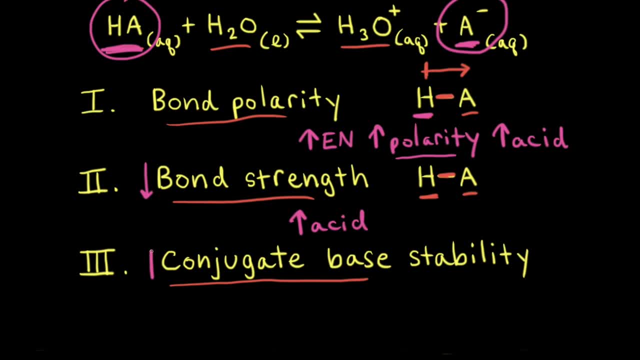 the stronger the acid. So let's go ahead and write here: an increase in the stability of the conjugate base means an increase in the strength of the acid, Even though acid strength is usually due to all three of these factors: bond polarity, bond strength. 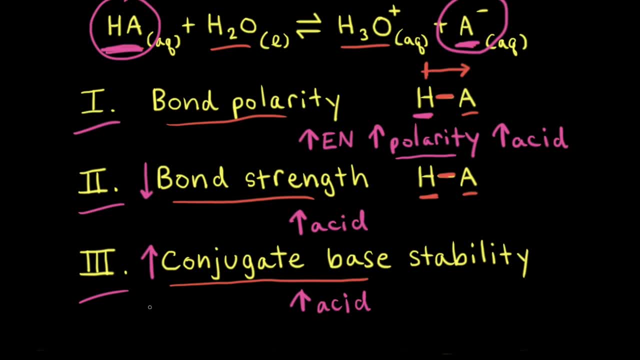 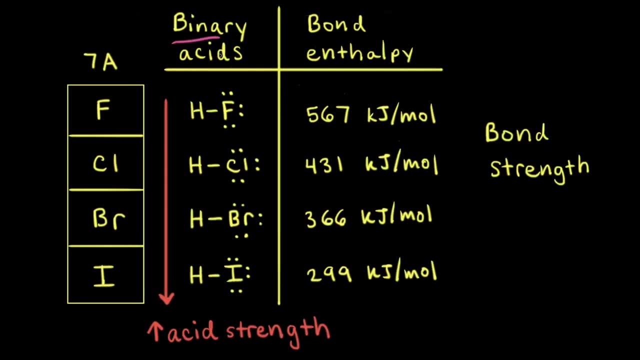 and conjugate base stability. when we look at examples, we're only gonna consider one or two factors that are the main contributors to acid strength. Let's look at the binary acids from group 7A on the periodic tables, That's hydrofluoric acid, hydrochloric acid. 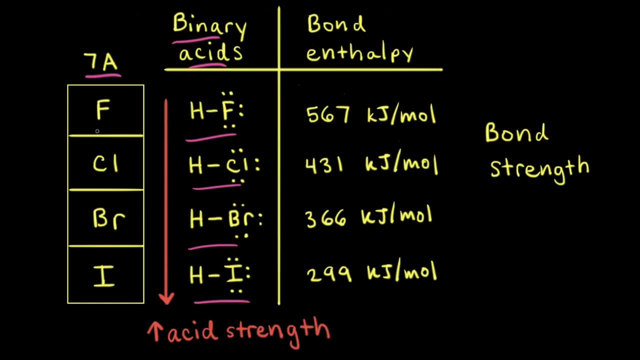 hydrobromic acid and hydroiodic acid. As we go down the group, from fluorine to chlorine, to bromine, to iodine, there's an increase in the strength of the acid. So out of these four, hydroiodic acid is the strongest. 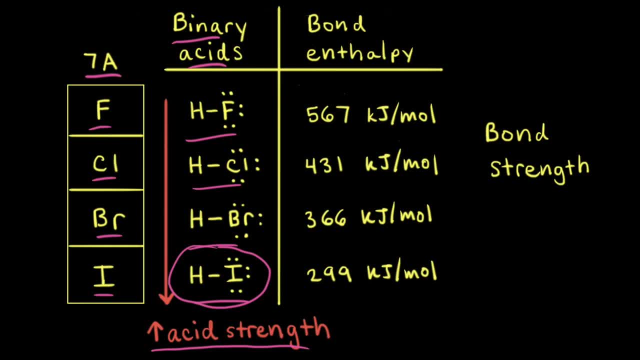 The main factor determining the strength of the binary acids in group 7A is bond strength. Looking at values for bond enthalpies allows us to figure out the strengths of these bonds. For example, the HF bond has a bond enthalpy of 567 kilojoules per mole. 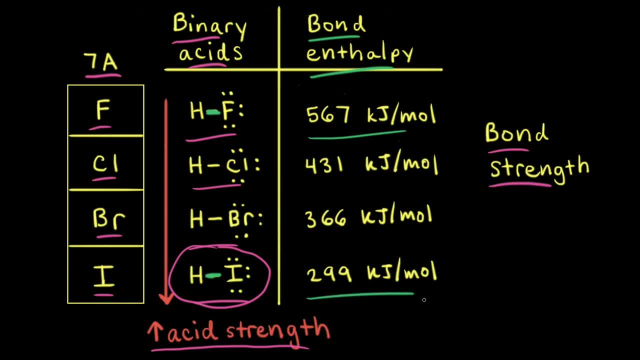 while the HI bond has a bond enthalpy of 299 kilojoules per mole For the value for the bond enthalpy, the easier it is to break the bond And because bond enthalpies decrease as we go down the group. 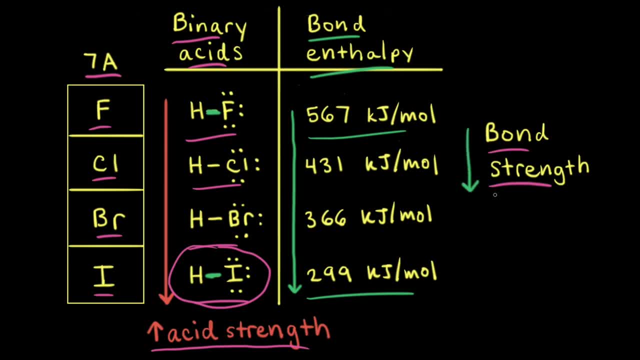 that means there's a decrease in bond strength. A decrease in bond strength means it's easier for the acid to donate a proton. Therefore, we see an increase in the strength of the acid as we go down the group. Next, let's compare the strengths of some oxyacids. 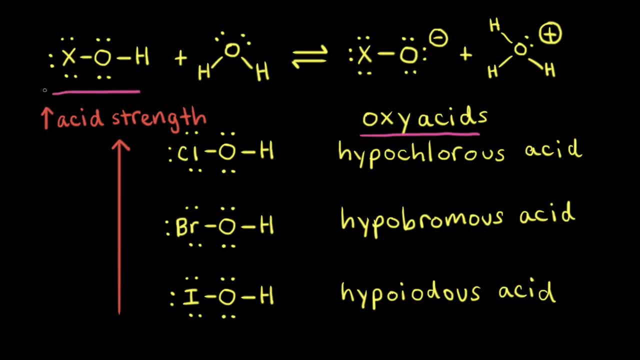 These oxyacids all have the general formula XOH. where X is a halogen, The acidic proton is the proton that's directly bonded to the oxygen, And if an oxyacid donates its proton to water, that forms the hydronium ion, H3O+. 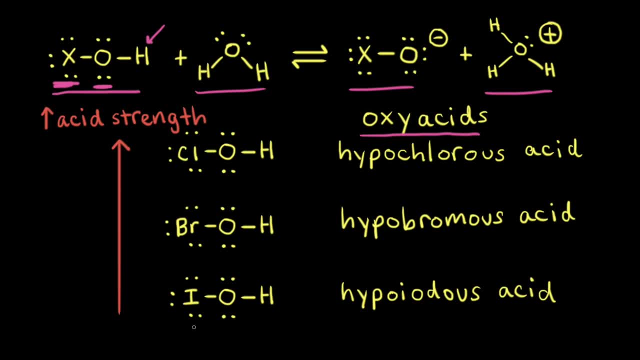 and the conjugate base to the oxyacid. For these three oxyacids, the halogens are iodine, bromine and chlorine, And as we go from iodine to bromine to chlorine in group 7A on the periodic table, 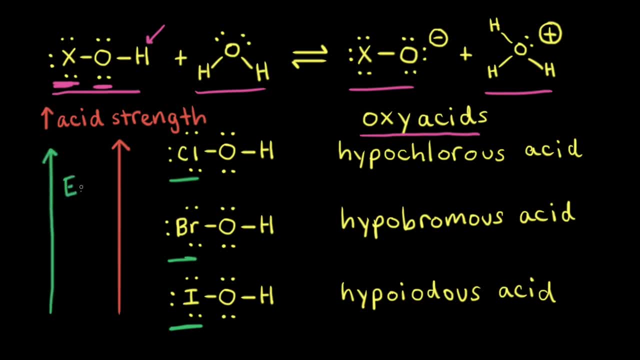 that's an increase in the electronegativity. So chlorine is the most electronegative out of these three halogens And as we go up the group in our halogens there's an increase in the strength of the acid. 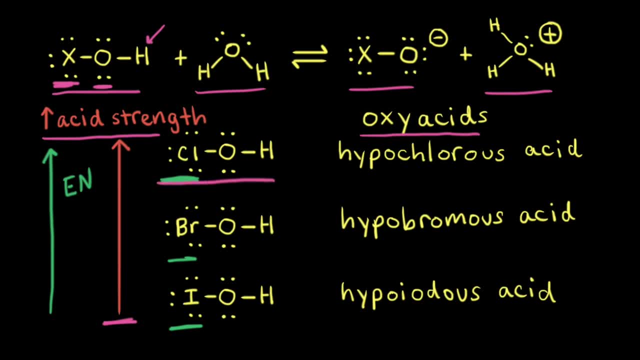 So hypochlorous acid is the strongest of the three. The main factor determining the strength of these oxyacids is the bond polarity, which is affected by the electronegativity of the halogen, So the polarity of this oxygen-hydrogen bond. 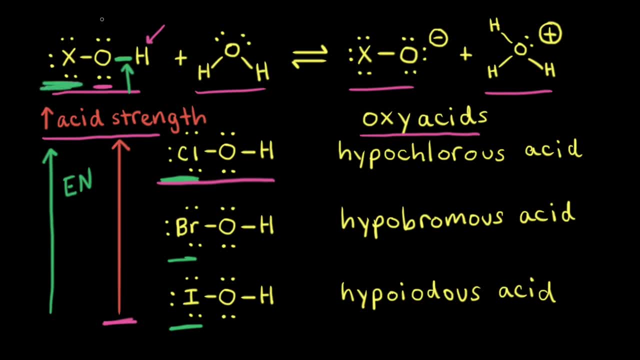 is affected by the presence of the halogen. As the electronegativity of the halogen increases, the halogen is able to withdraw more electron density away from the right side of the molecule. That increases the polarity of the OH bond. 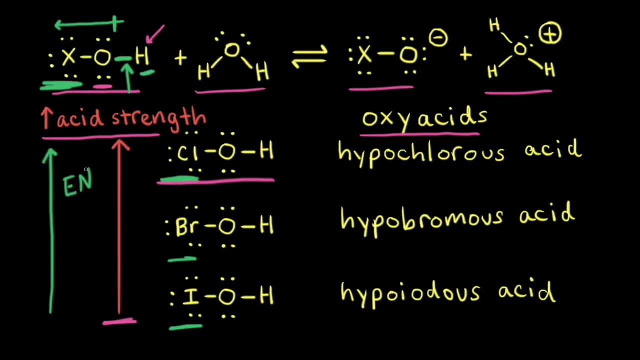 It makes it easier to donate this proton. Therefore, as the electronegativity of the halogen increases, the acidity of the oxyacid increases. This effect of the electronegative atom increasing the acidity is often referred to as the inductive effect. 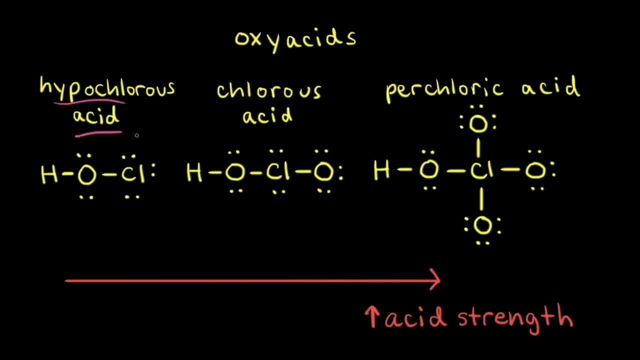 Let's compare hypochlorous acid to two other oxyacids And notice how I've left the formal charges off of these acids just so we can focus on general structure. Notice how the acidic proton is directly bonded to the oxygen in all three of these oxyacids. 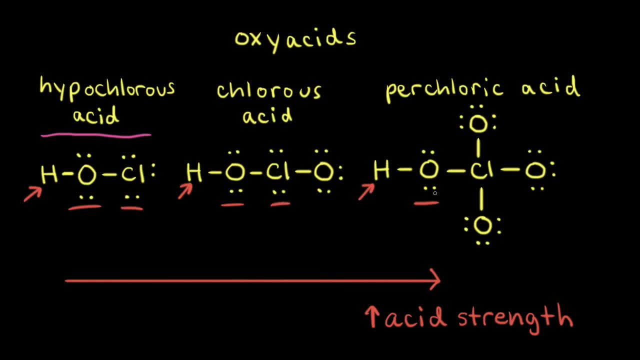 And in all three of these oxyacids the oxygen is directly bonded to a chlorine. Notice what happens to the structure as we move to the right, Comparing chlorous acid to hypochlorous acid. chlorous acid has an additional oxygen. 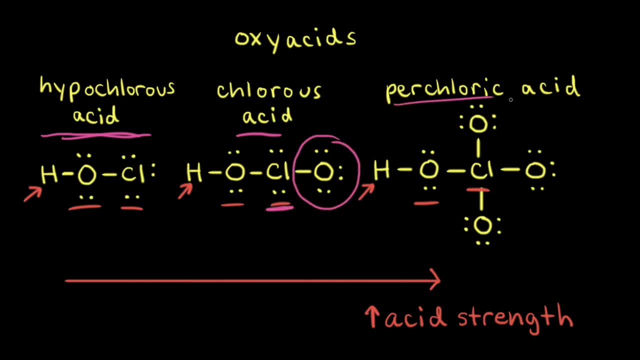 bonded to the chlorine And looking at perchloric acid, instead of only one additional oxygen, there are three additional oxygens. So as we move to the right, we're increasing in the number of oxygens bonded to the chlorine. Oxygen is a very electronegative element. 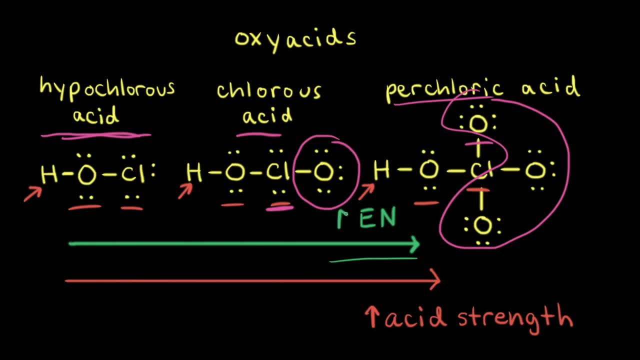 So as we move to the right, we're increasing in the number of electronegative atoms in the acid, And as the number of electronegative atoms increases, more electron density is pulled away from the acidic proton, which increases the polarity of the oxygen-hydrogen bond. 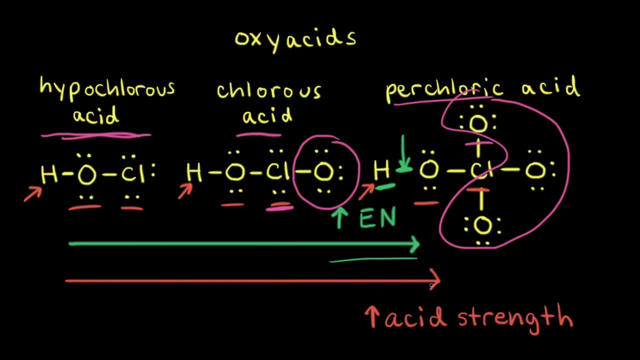 So bond polarity increases as we move to the right, which predicts an increase in the strength of the acid as we move to the right, And that's what we observe experimentally. Perchloric acid is the strongest of the three. In reality, all three factors. 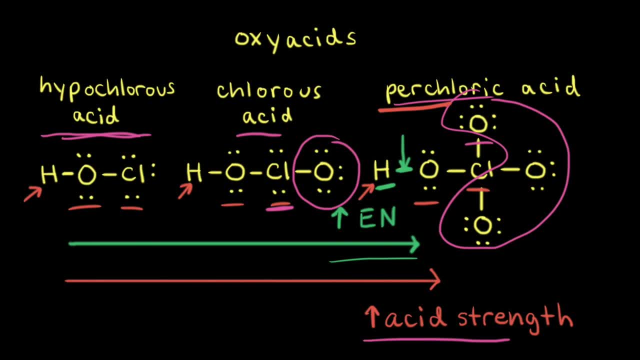 affect the strength of the acid. However, for simplicity's sake, we could just say that increasing bond polarity is the main factor for the increasing acid strength in these oxyacids. Carboxylic acids are a group of acids that all contain a carboxyl group. 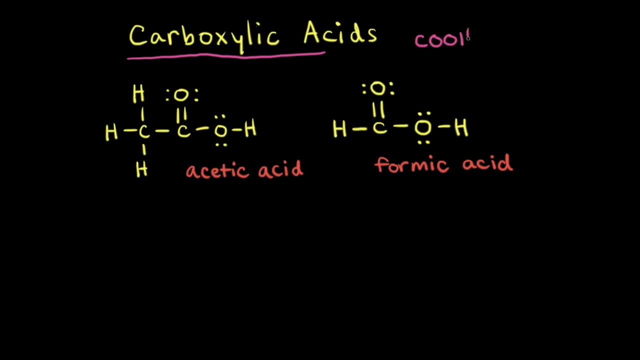 A carboxyl group consists of carbon, oxygen, oxygen and hydrogen. So if we look at acetic acid, I'll circle the carboxyl group on acetic acid and I can also circle the carboxyl group on formic acid. 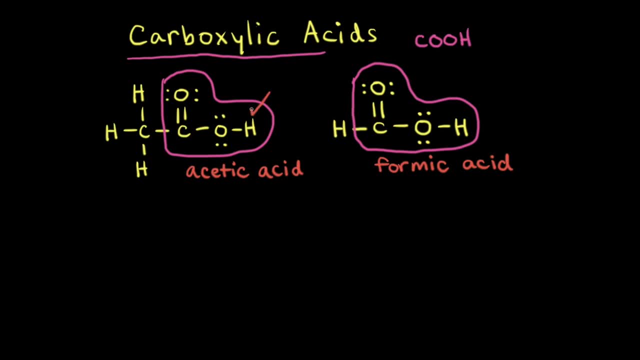 The acidic proton in a carboxylic acid is the one that's directly bonded to the oxygen in the carboxyl group. One reason why this proton is acidic is because of the presence of this oxygen in the carboxyl group. This oxygen-hydrogen bond is already polarized.